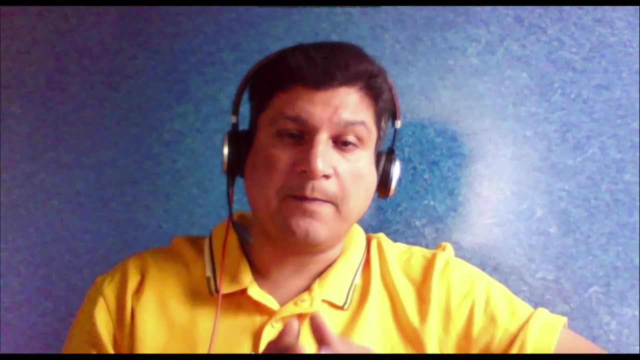 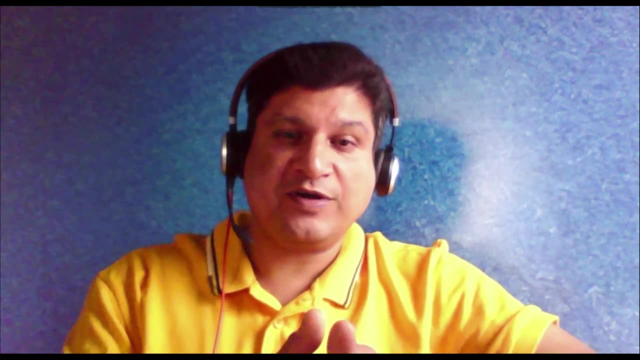 Friends, I'm creating a lot of quality contents for you, but I'm not getting subscribers. I want you to like, share and subscribe my channel so that I can grow Code One Digest family. Thank you, All right, let's get started. So let's start with the Memento Design Pattern. 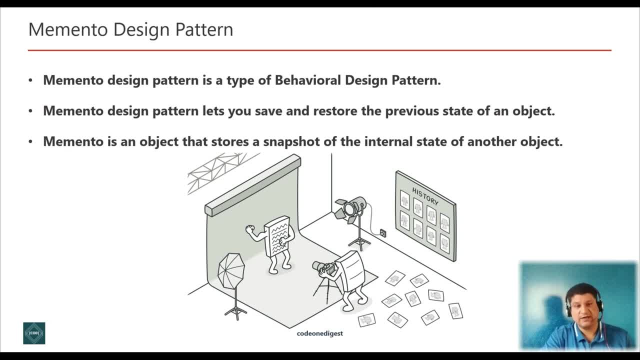 Memento Design Pattern is a type of behavioral design pattern that lets you save and restore the previous state of an object without revealing the detail of its implementation. A Memento is an object that stores a snapshot of the internal state of another object. This pattern, 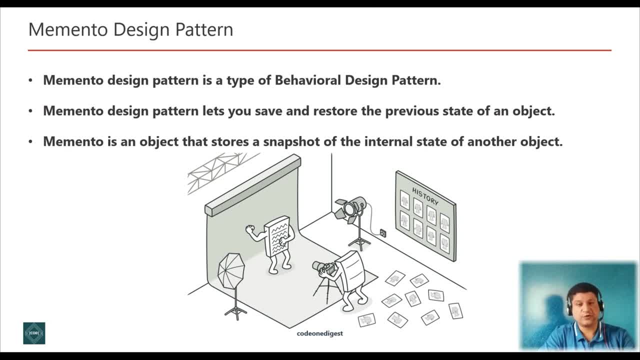 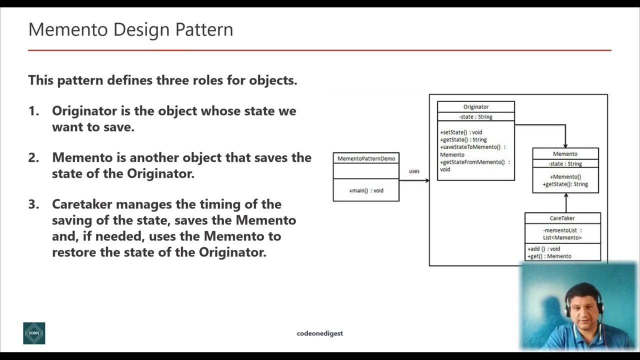 allows you to save the internal state of an object to restore it later. Let's take an example: In your application is growing, progressing, You may want to save a checkpoint in your application and restore it back to the previous state if anything goes wrong. Right, This pattern defines three roles for an object: Originator, Originator. 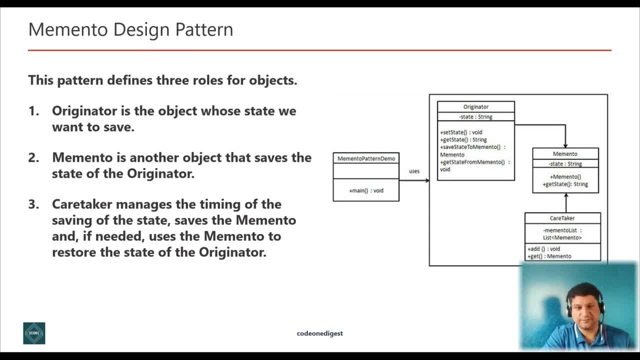 is an object whose state will be saved- Memento. Memento is another object that saves the state of an originator object. And third is Caretaker. Caretaker manages the timing of saving the saved by the memento and, if needed, uses the memento to restore the state of the 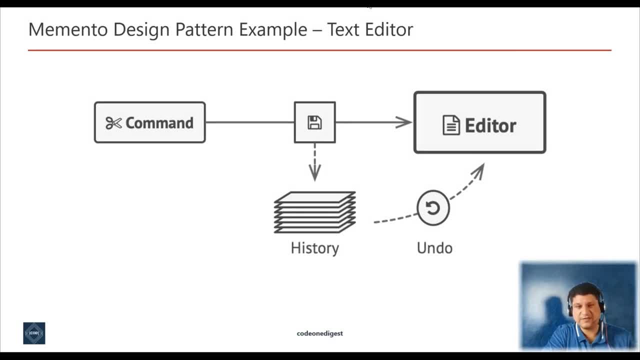 originator. let's discuss an example now. imagine that you are creating a text editor app. in addition to simple text editing, your editor can format text, insert inline images, etc. at some point, you decide to let user undo any operation carried out on a text. for this implementation, your app should record: 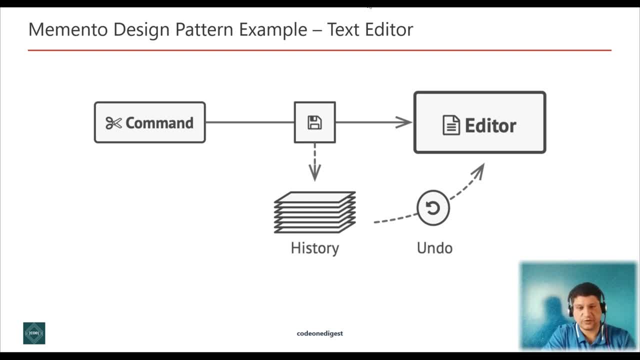 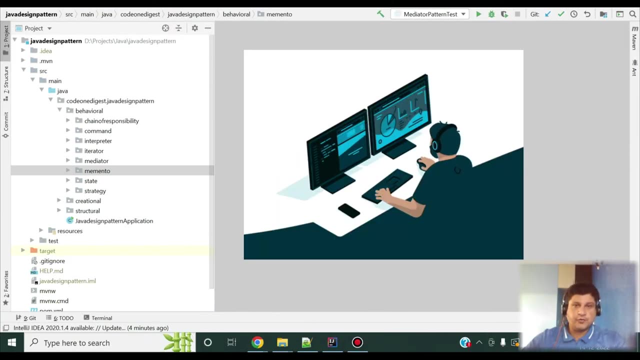 the states of all the objects and save it in some storage. later, when user decides to revert an action, then app fetches the latest snapshot from the history and use it to restore the state of all the objects. friends, I have prepared a code snippet for the memento design pattern. let me show you the code. 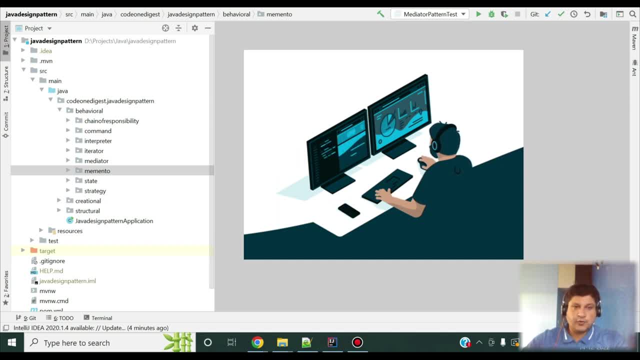 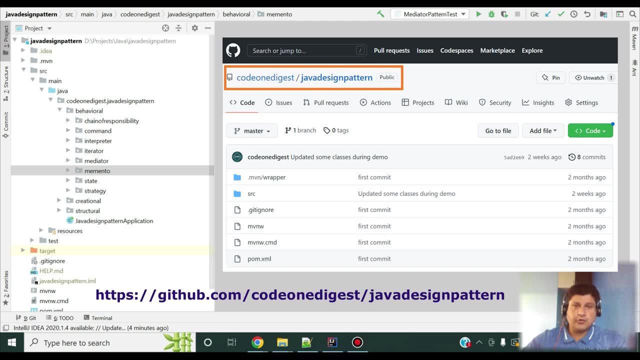 and then I'll run this code and give you the demo of memento design pattern. friends, this code is available in my gallery and you can download it from the library and download it from your github repository. you can download and play with it. the link of github. 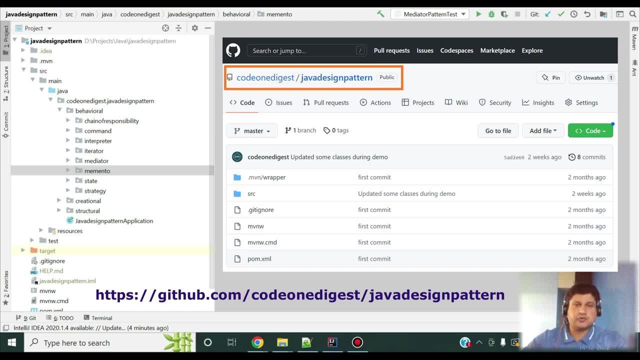 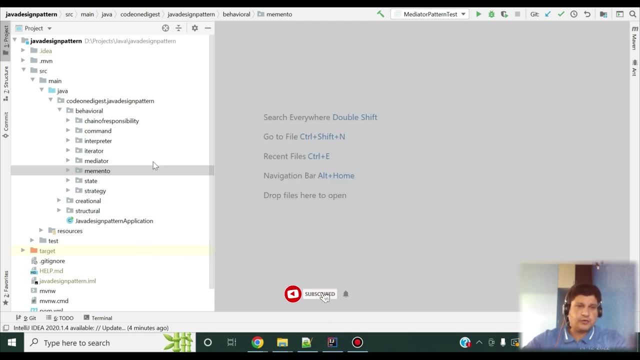 repository is shown on the screen and also shared in the description section of this project. okay, now let me show you what I have done. so I have a package memento where I have all my classes. then, as I said, in memento we have three component, three actors in the memento design pattern one: 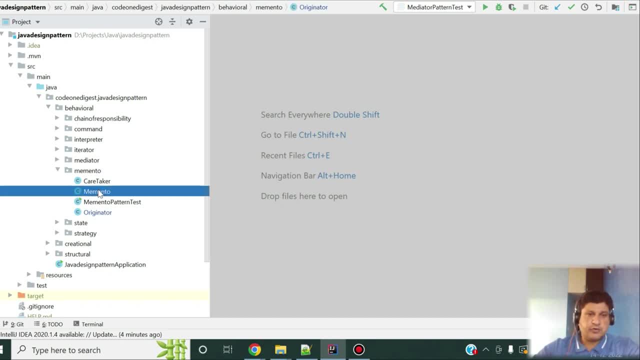 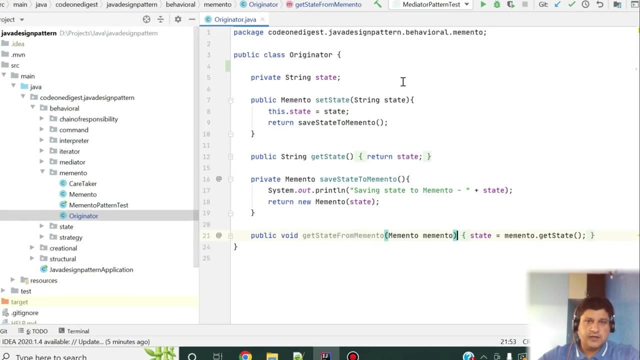 is originator. this is our context, is our memento object which keeps a state of originator, object and caretaker, caretaker, maintain the lifecycle of all the states. so let's see the originator first. originator is our context. it has a string called state and then it has 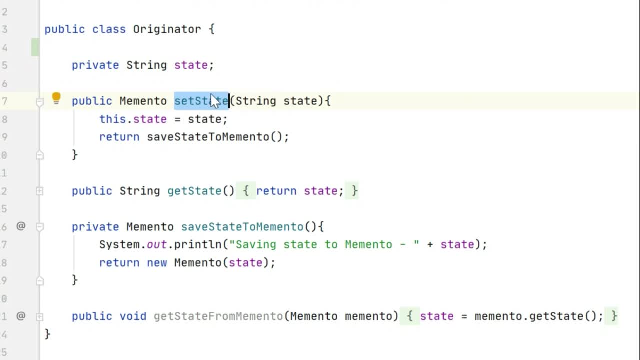 method to set a state. we are setting the state here and in this set method we also saving that state to the next state. here you can also save any of the state to memento. then we have a method called get state. it will give you the state and save. 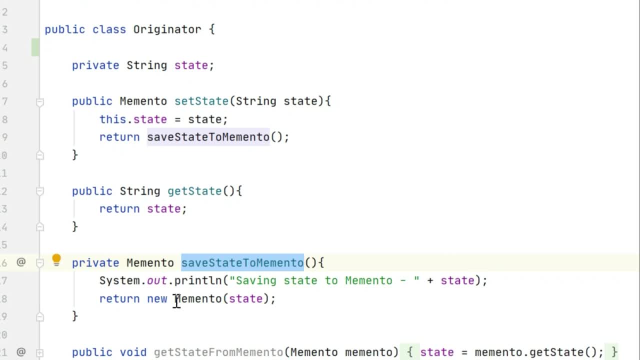 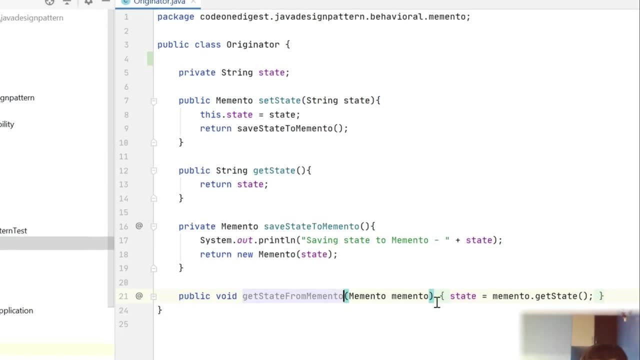 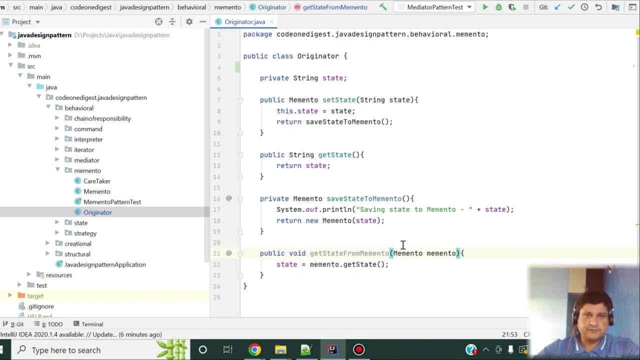 state to memento. in this method we are creating a object of new memento, passing the state and saving it. then we have another method: get state from memento, so we can get the state from memento and return it. then we have a memento. this is where we are actually. 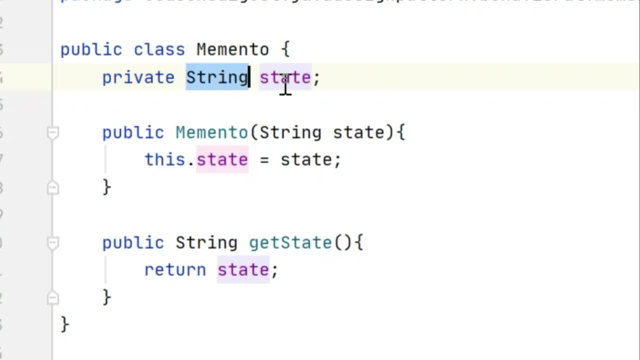 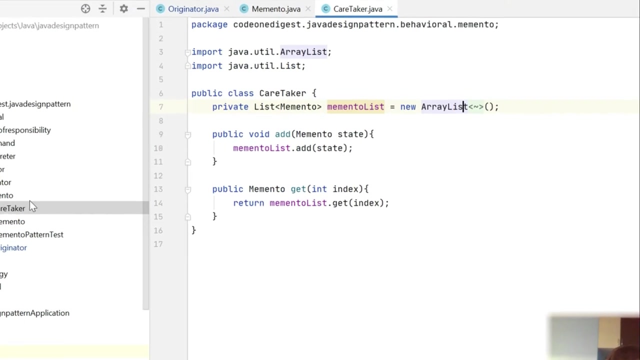 saving the state of an object. we have string state we are. we are having a constructor of memento where we are initializing this state through this constructor. we have a get state method where we are returning this state. right now, let's see a ktacker. in ktacker we have 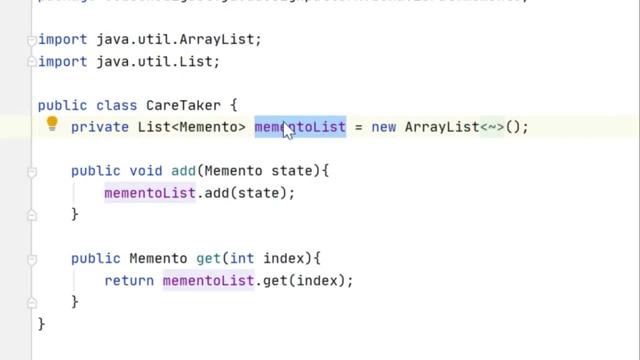 a list of memento objects. so this is where actually we are having the records of all our states, all of our mementos. then we have method here: add in add, we are adding, we are passing the state and we are saving that state to this list. 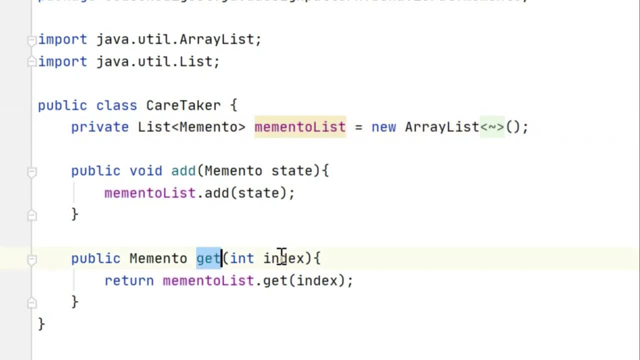 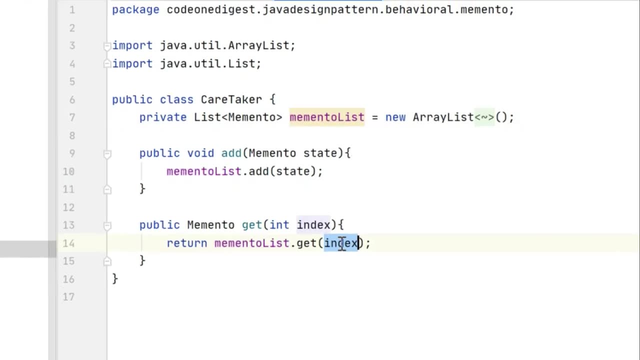 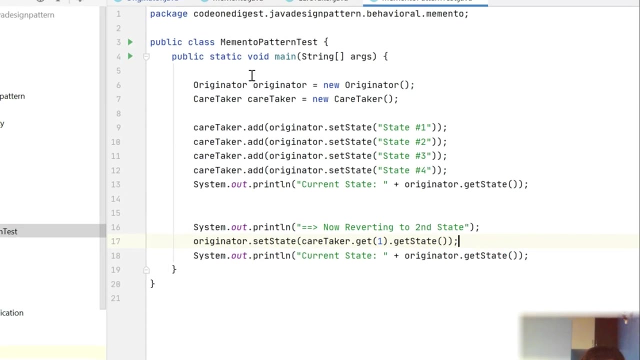 and get state. here in this get method we are passing a index and we are returning the memento object from this list based on that index. i have also written a test class. let's see how the test class looks like. so in this test class i am initializing one originator object. 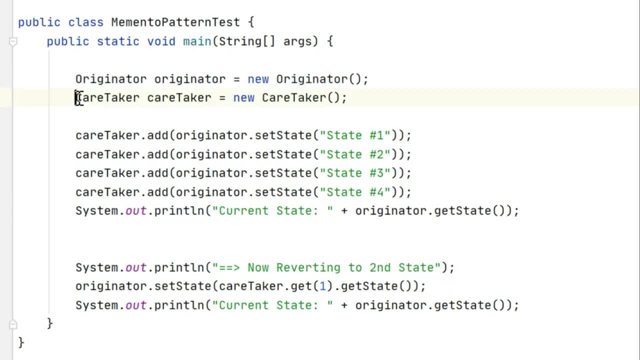 this is our context. then i am initializing one ktacker object and then i am calling ktacker dot add method where i am setting a new state. i am saying originator dot set state state one, then state two, state three. this method returns me an object of memento. this methods returns me. 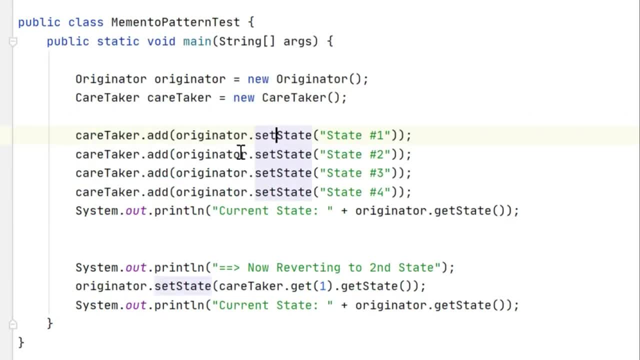 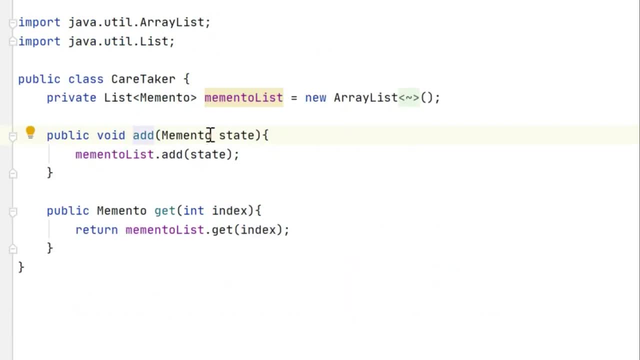 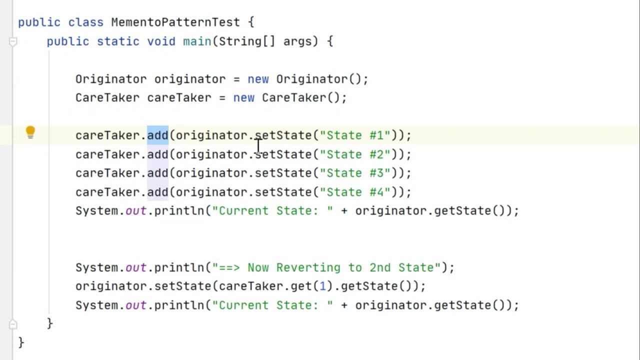 an object of memento and that's what we save: that object into our list. this add method. add method: adding that state, adding that memento state to this list. right, we are doing that. we are saving all the state as we are changing the originator object. we are keep saving this. 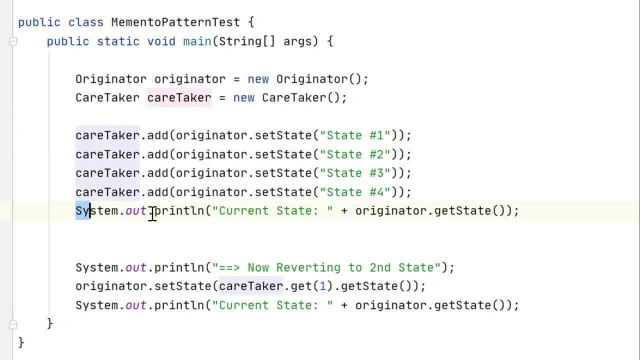 state into ktacker. and here we are at this moment we are printing what is my current state and then i want to revert this state of my originator object to second state. so what i am doing is originator dot set state, ktacker dot get set state, other state i am. 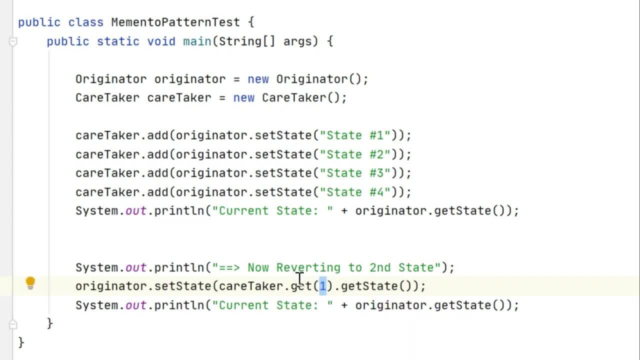 get one dot- get state. so this get method takes a index and it returns an object of memento and memento is having a state string. that is what we are getting from this method- get state- and we are setting that state into originator set state and this is that is how our originator revert back to. 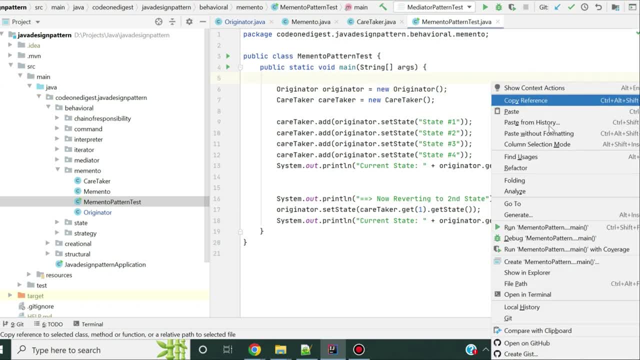 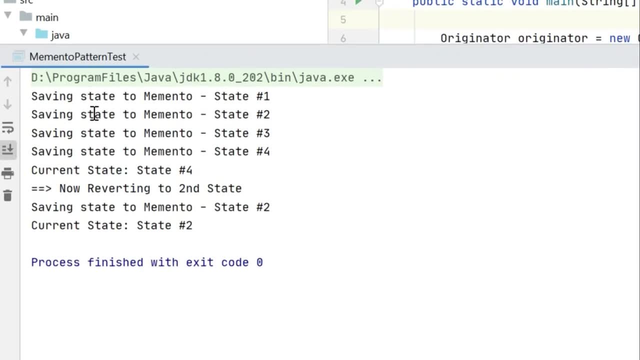 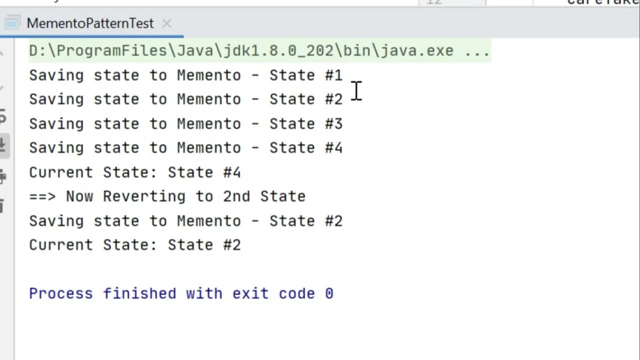 the second state. let me run this and show you how that works: compiling the code. yeah, there you go. so it says: when we are saying: when we are saving the state one, two, three, four. it says saving state one, two, three, four and so on. and then we are printing: what is my current state? it says: 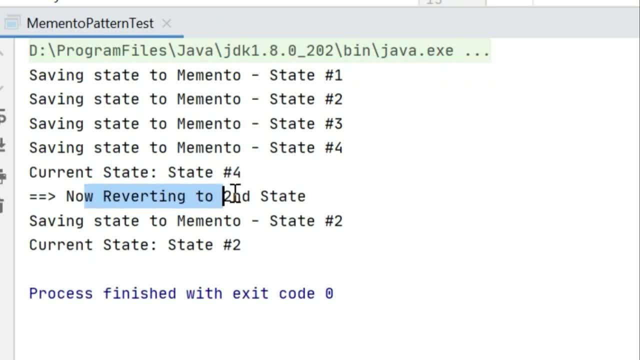 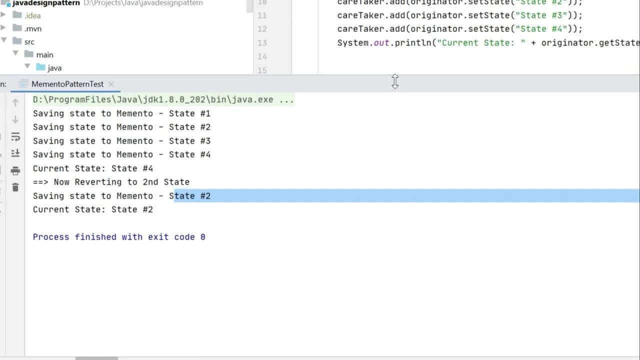 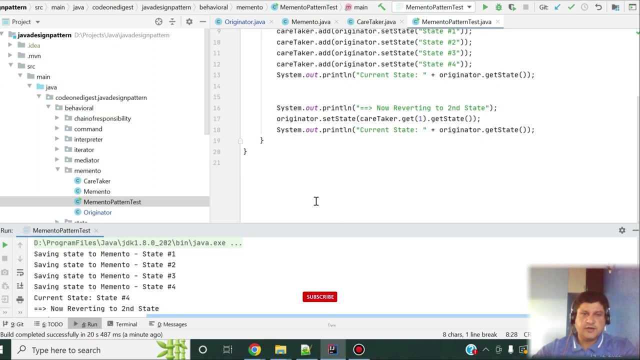 my current state is four. now i'm reverting to a second state, so after saving, i'm printing that, saving this state to state two, then my current state becomes state two. so this is a very simple example. this is a very simple implementation of memento pattern, where you keep saving the state of your originator object. 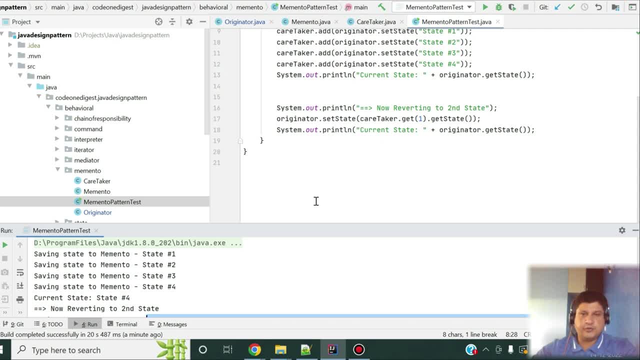 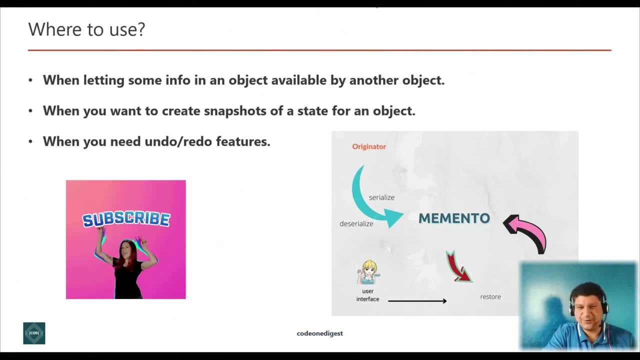 and you can revert back anytime you want to to the previous state, right? okay, friends, the very first question comes to our mind: where to use memento design. okay, friends, the very first question comes to our mind: where to use memento design pattern. so you can use memento design pattern when you want to let some info in in the object. 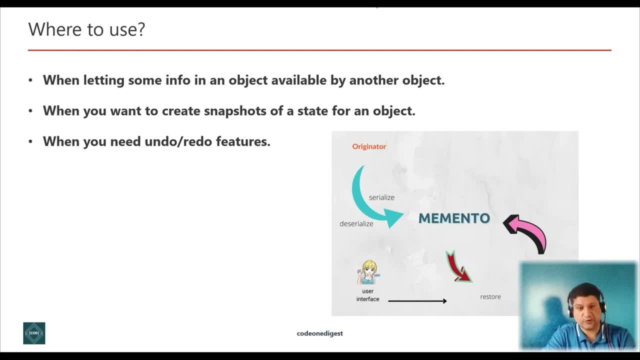 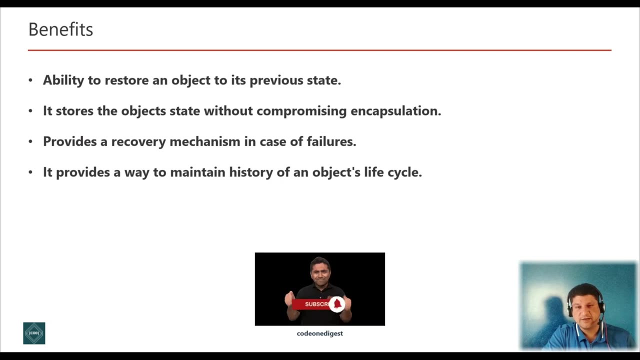 available by another object. when you want to create a snapshot of the states of an object and when you need to redo undo feature in your application, that time memento pattern can be used right. so what are the benefits of the memento design pattern? it provides you ability to restore an object to its previous state. it stores the 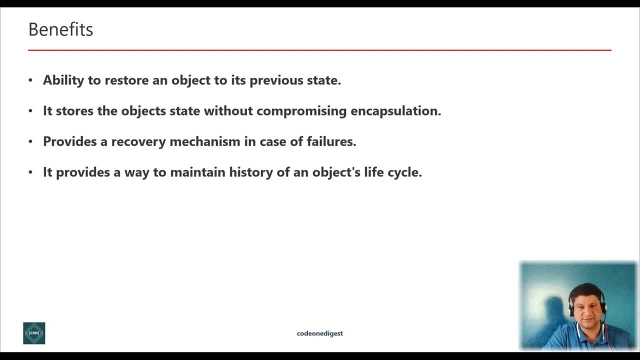 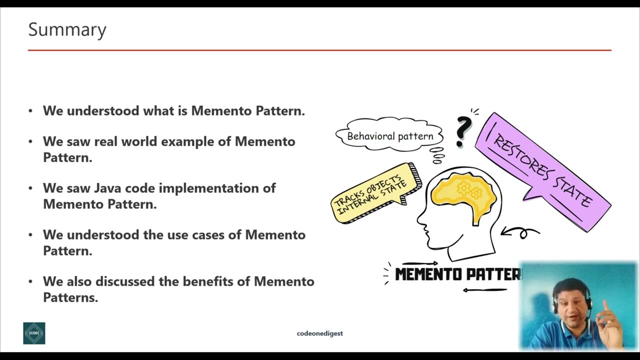 object state without compromising the encapsulation, and it provides a recovery mechanism in case of failure. it provides a way to maintain history of an object's life cycle, right, okay, friends. now let me summarize what we learned in this video. we understood what is memento design pattern. 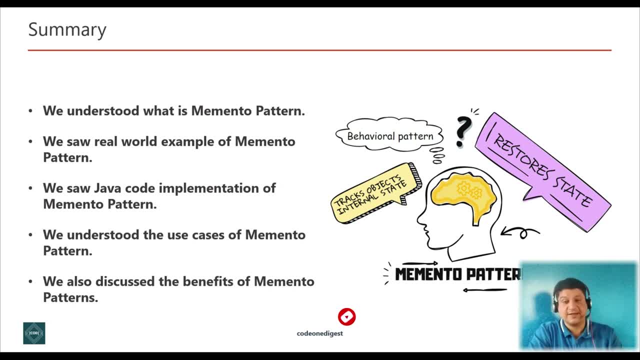 we saw a real world example of memento design pattern. we also saw java code implementation of memento design pattern and we also saw use cases of memento design pattern and at the end, we discussed the benefit of memento design patterns. right, friends, let me know if you have already used. 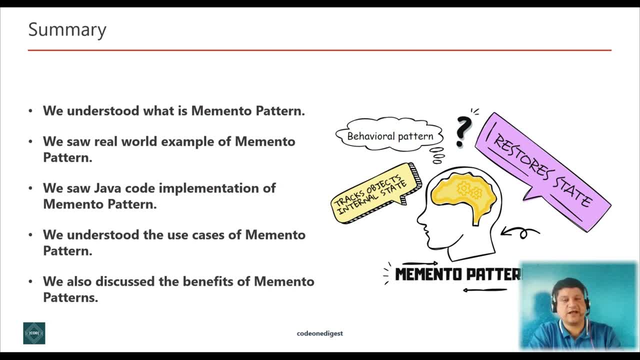 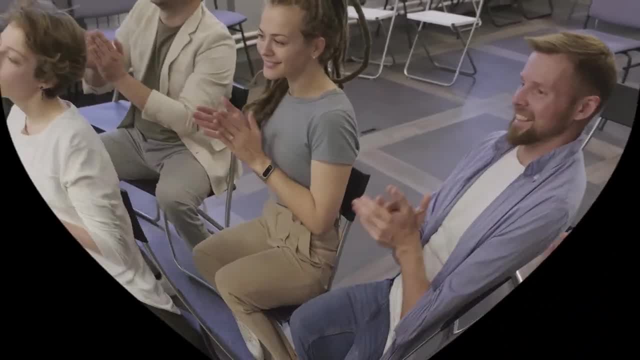 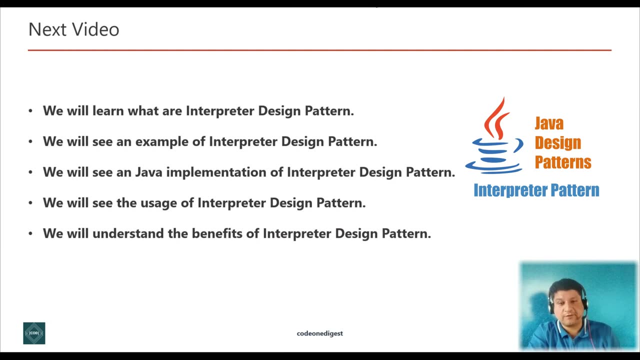 the memento design pattern in your project or seen a scenario where this pattern can be very useful? please provide your answer in the comment section. you the next video. we will cover interpreter design pattern. we will learn what is interpreter design pattern. we will see the usage of interpreter design pattern. we will see java implementation. 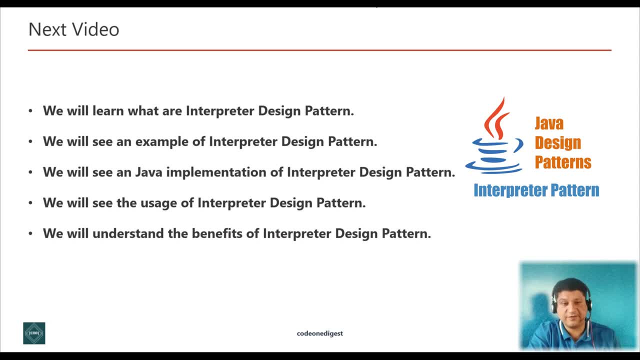 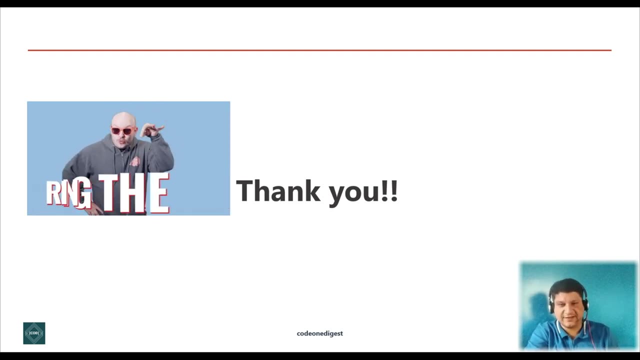 of interpreter design pattern and we will understand the benefits of interpretation design pattern. so stay tuned for the next video and please subscribe to this channel to grow our code one digest family friends. i request you to subscribe to the code one digest channel for the latest programming and technology related videos. i am putting a lot of efforts.